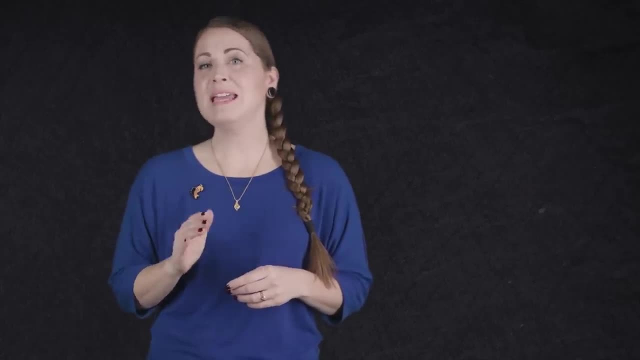 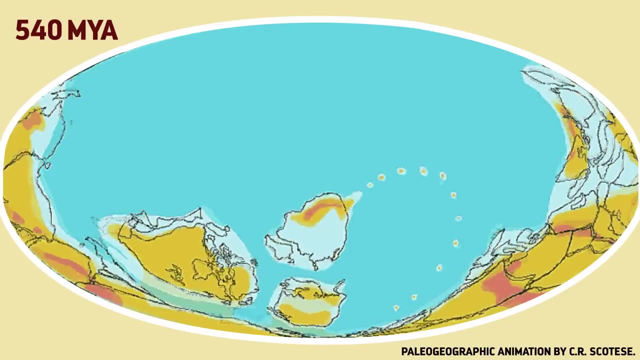 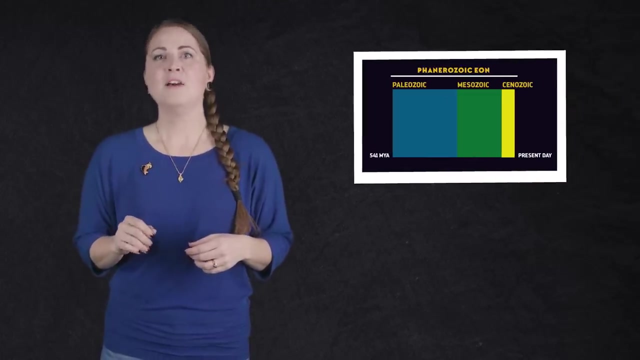 But the fact is, the Paleozoic Era was truly a make-it-or-break-it time for life on Earth. At the beginning of the Paleozoic, living things were extremely simple and not very dynamic. Life was fragile, vulnerable. But the Paleozoic was also easily the most chaotic of all three eras of our eon, with 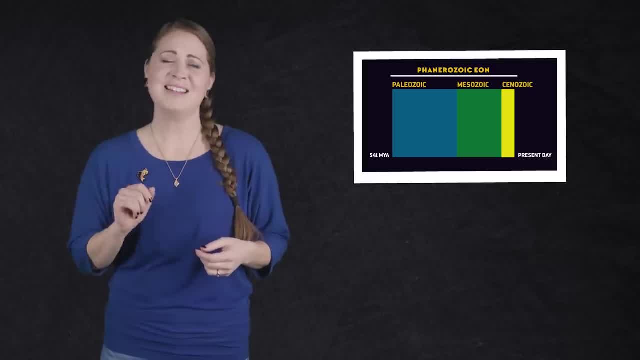 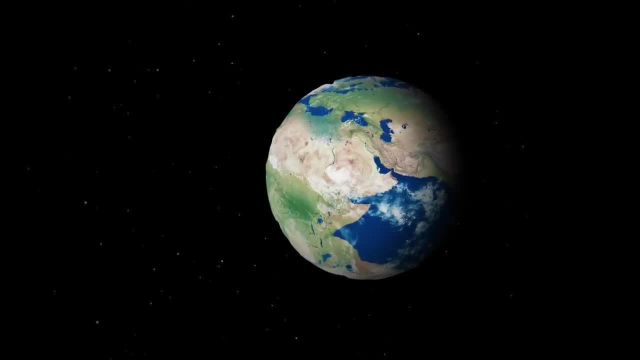 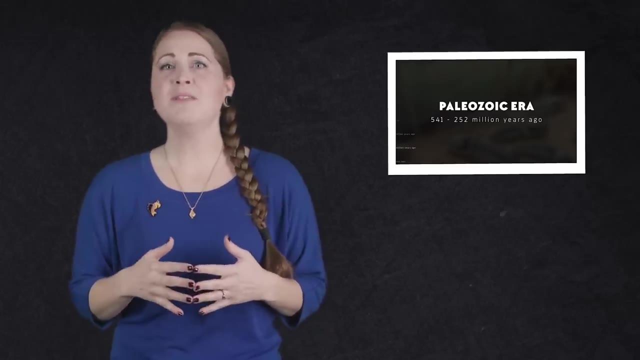 near-constant revolutions in life. In fact, by the end of this era, our planet was the closest it's ever gotten to being devoid of life altogether. It's the closest that life ever got to just failing So far from dull. the Paleozoic Era just might be one of the most harrowing chapters in the 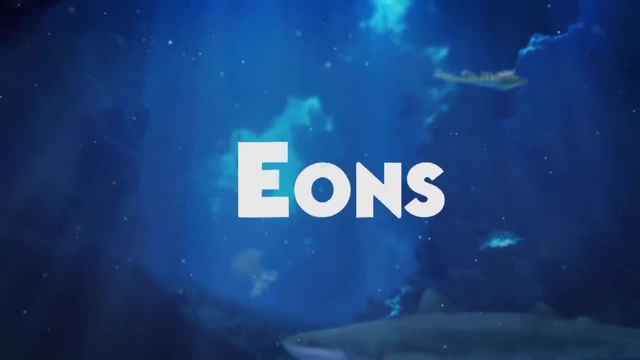 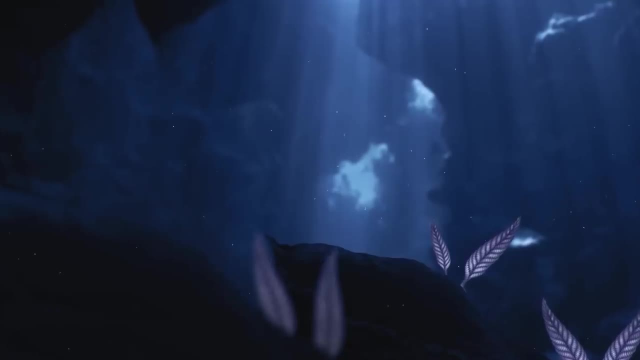 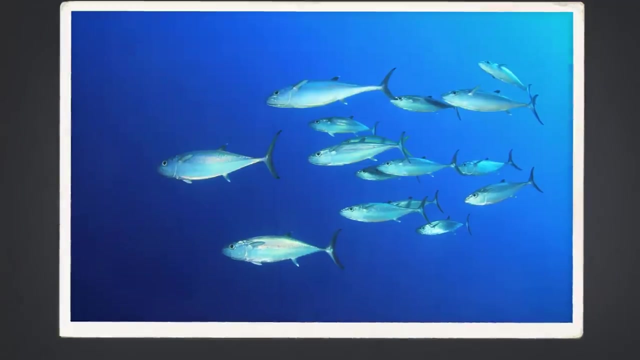 story of life on Earth. For the first three and a half billion years or so that life existed on this planet, things were simple. Almost all living things were in the oceans and most of them couldn't move on their own. So the big, complex ecosystems that we know today, with active predators and mobile prey- 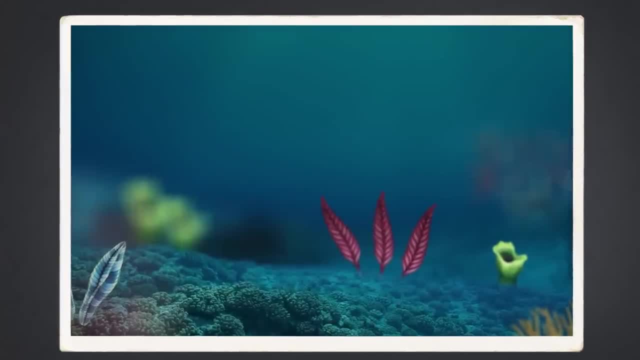 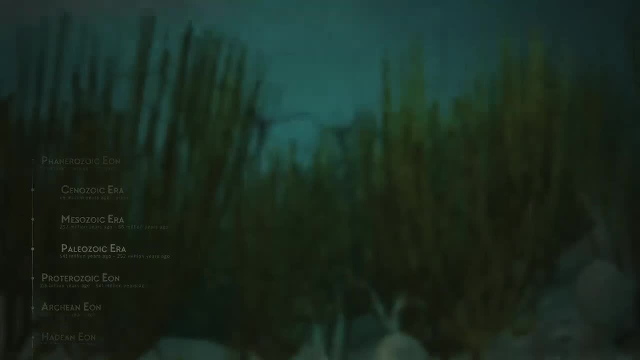 didn't really exist. Pretty much whatever drifted by you was what you ate. That is until about 541 million years ago, when the Paleozoic Era began, with a period known as the Cambrian, And right from the start things were dramatic. 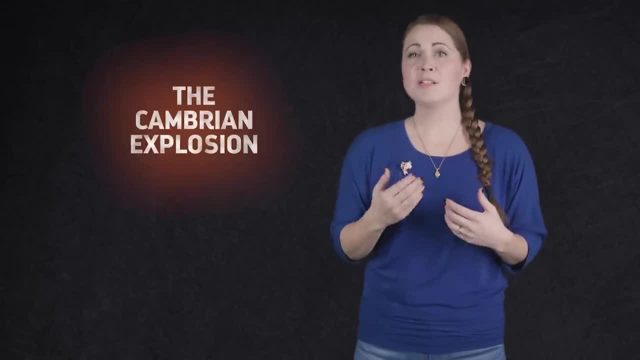 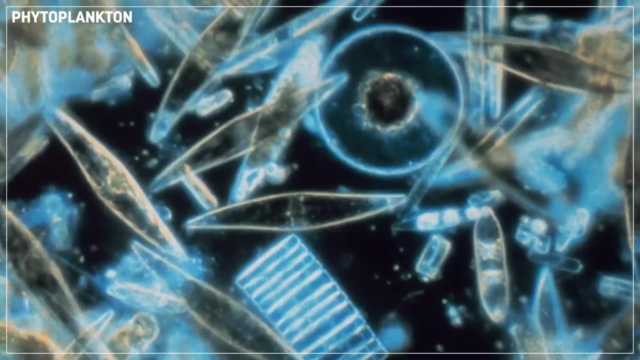 This burst of evolutionary innovation, which you know as the Cambrian Explosion, was likely the result of a whole bunch of environmental triggers. In the early Cambrian, thanks to a boom among phytoplankton and salmonella, there was a rapid rise in oxygen levels in the oceans, allowing life to flourish. 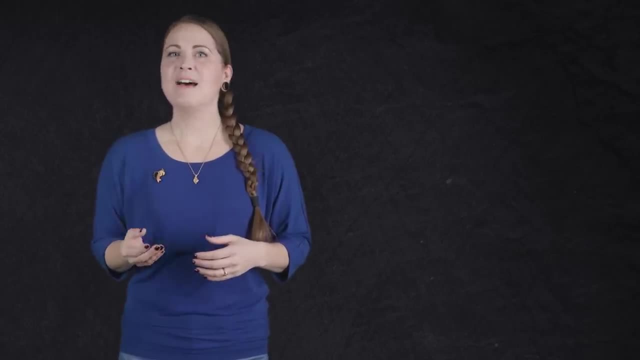 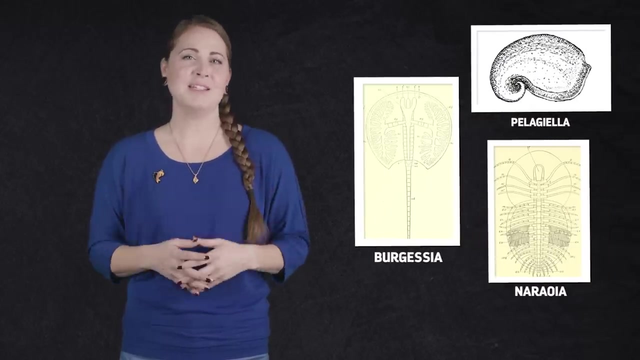 Meanwhile, changes in the chemistry of the oceans brought on by erosion allowed animals to develop things like shells and exoskeletons, and this led to the formation of new body plans that the world had never seen before. Almost every major group of animals that exist today developed within the first 40 million. 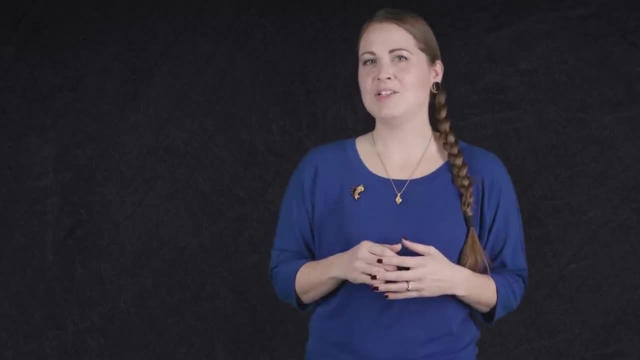 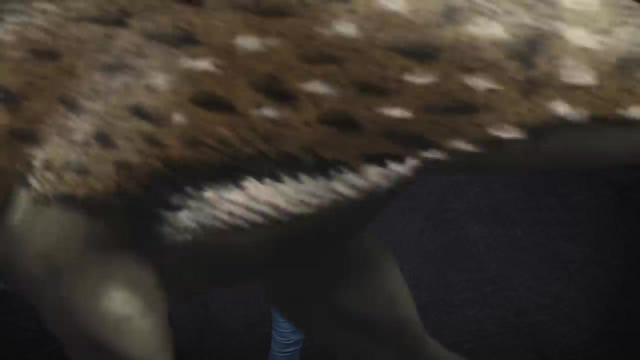 years of the Cambrian, along with many game-changing adaptations like calcified heart parts, flexible limbs and the very first eyes. For instance, the first large-bottomed cambrian, which was the first large-bottomed cambrian, was the first to develop a large, large predatory organism like Anomalocaris, which hunted worms and other soft-bodied creatures, And over time, some animals, like arthropods, developed hard exoskeletons to protect themselves, But others, like pikaia and haikuela, went in a different direction. They developed the ability to swim under their own power with a flexible rod of cartilage. 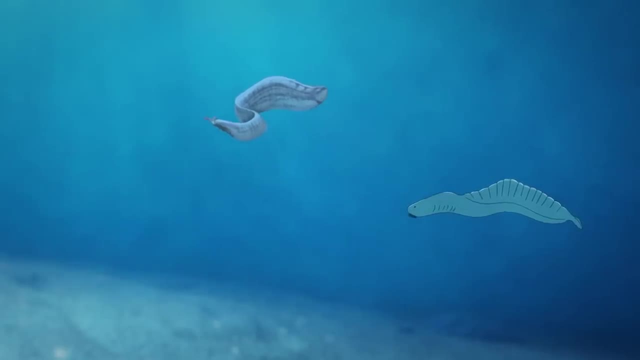 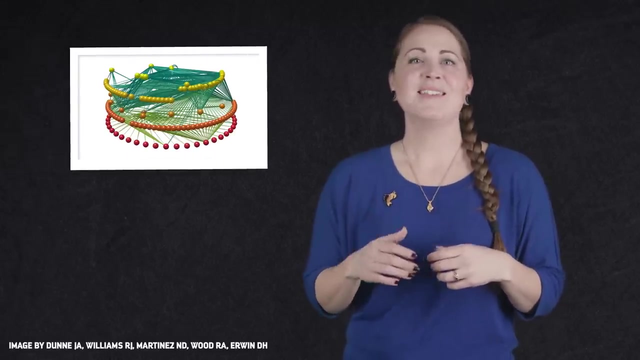 to power their tail. These ancient swimmers would become the ancestors of the vertebrates. Major breakthroughs like these resulted in whole new fantastic ecosystems with complex webs that life had not experienced before. But this explosion of life couldn't last forever. 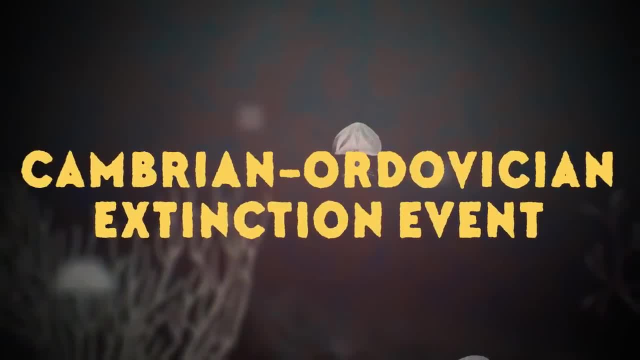 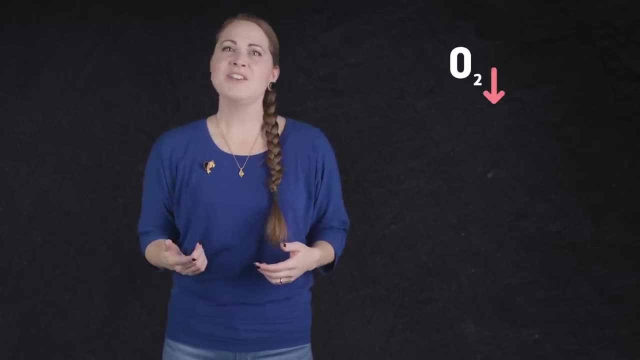 The Cambrian ended 488 million years ago in a mysterious mass extinction that saw the disappearance of many trilobite and mollusk species. While this extinction is not well understood, a sudden crash in oxygen levels may have been to blame, And remember that, because a lot of the pivotal events in the Paleozoic will hinge on the amount. 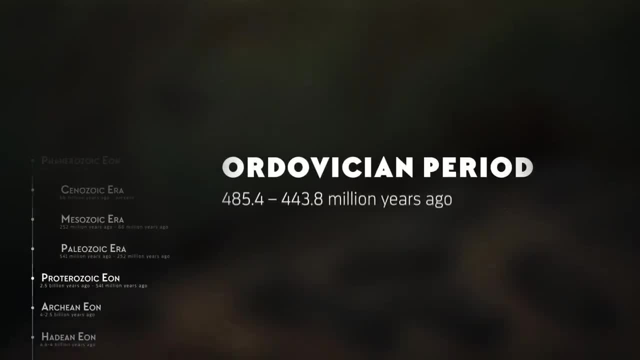 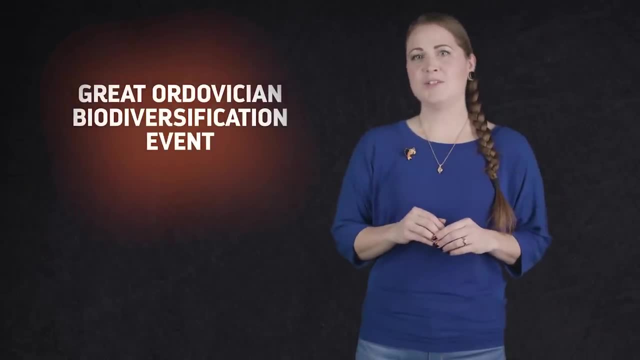 of oxygen, either in the oceans or in the atmosphere. But the next period, the Ordovician bounced back with another burst in diversity. This one's known as the Great Ordovician Biodiversification Event, or GOBE. You can think of the GOBE as kind of the sequel to the Cambrian Explosion, a sequel that was. 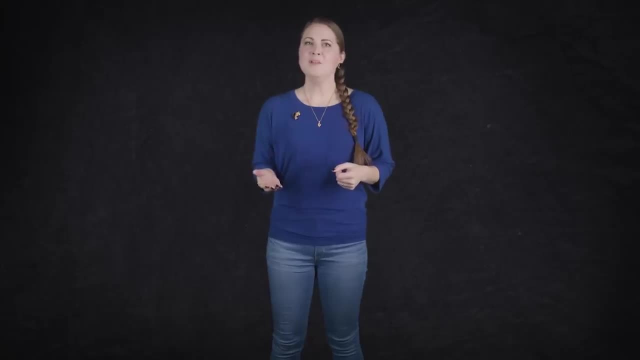 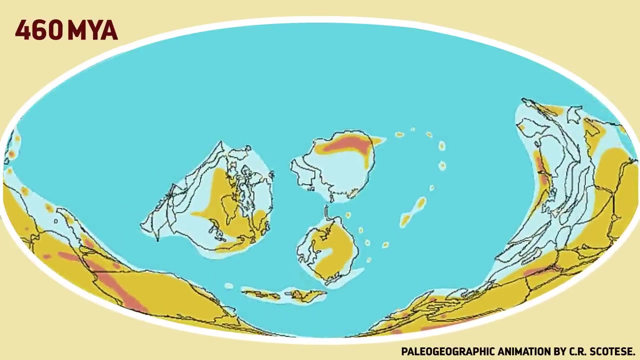 every bit as impressive as the original. Like the Cambrian event, the GOBE was brought on by a host of changes in the environment. For one thing, a burst of geological activity about 470 million years ago meant that the continents were on the move, creating new chains of islands and, with them, new isolated 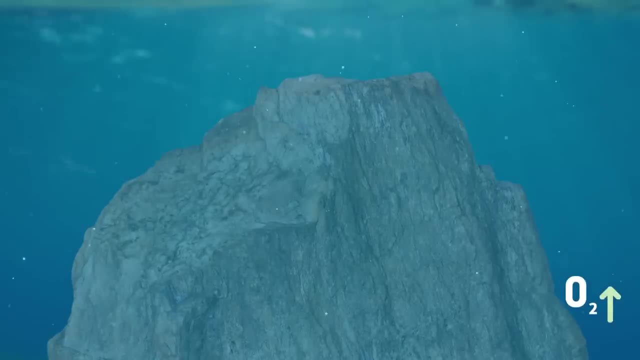 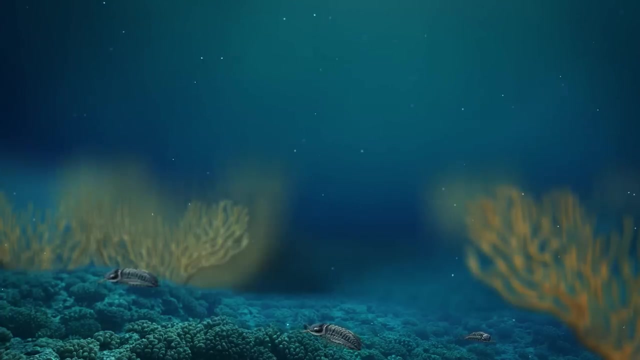 habitats And this, combined with changes in sea level and another change in water quality, led to a change in the environment, And then another boost of oxygen in the oceans stimulated a lot of rapid change. For example, this is when the first true fish appear on the scene, ostracoderms, which were 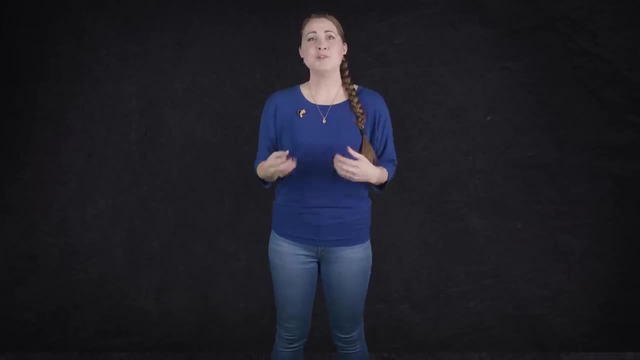 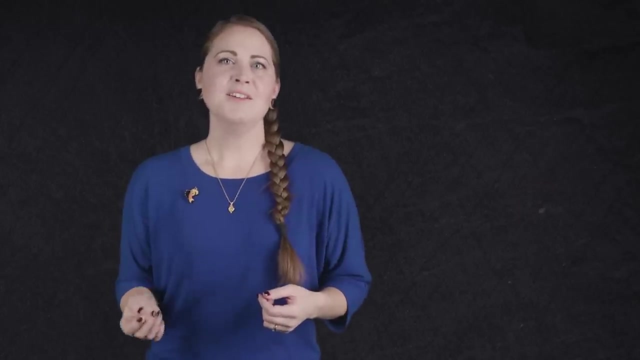 jawless and covered in bony plates. Meanwhile, cephalopods reached new lengths, like the shelled giant Camarasaurus, which grew up to 6 meters long. But while all this was going on in the water, things on land were truly revolutionary. Before the Ordovician, terrestrial life was probably limited to microbes, but early in the GOBE, the very first land plants sprouted in the primordial rocks, Based on their fossilized spores. we know these plants were small like modern mosses. 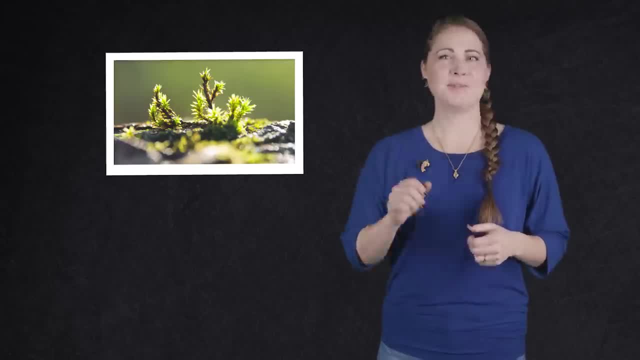 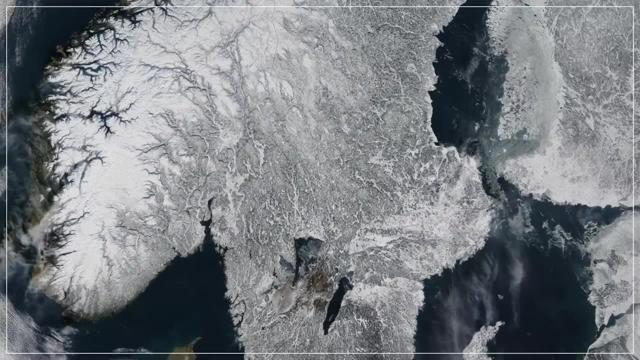 And, if anything, this early greenery might have been too successful. The massive number of plants on land took in so much carbon dioxide that the Earth's temperature plummeted And boom ice age. This cold snap occurred 444 million years ago, just as marine oxygen levels started. 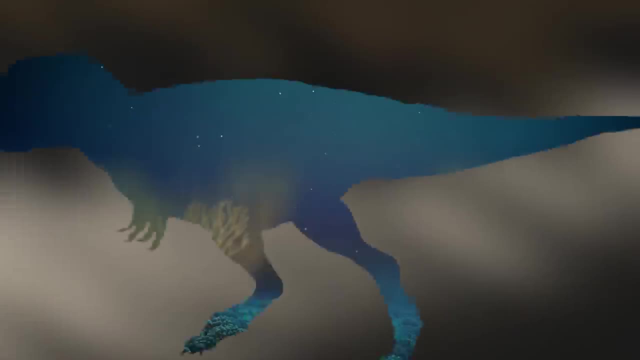 to drop, And this combination caused the most devastating mass extinction that animal life had faced so far. The Ordovician-Solarian extinction event wiped out 86% of the world's life, And that's why we're here. Thanks for watching. 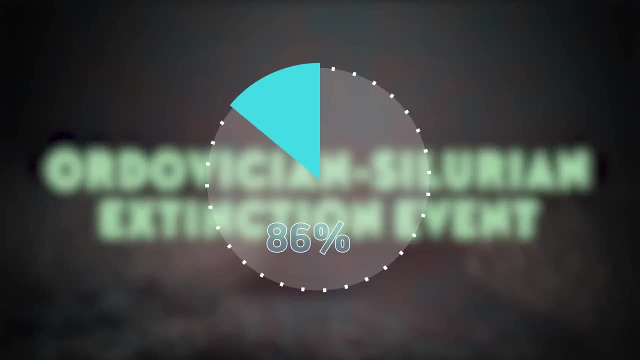 If you enjoyed this video, be sure to give it a thumbs up and subscribe to our channel for more videos like this one, And don't forget to turn on your notifications so you don't miss out on any of our latest videos. As you can tell from the name, it brought an end to the Ordovician and marked the beginning. 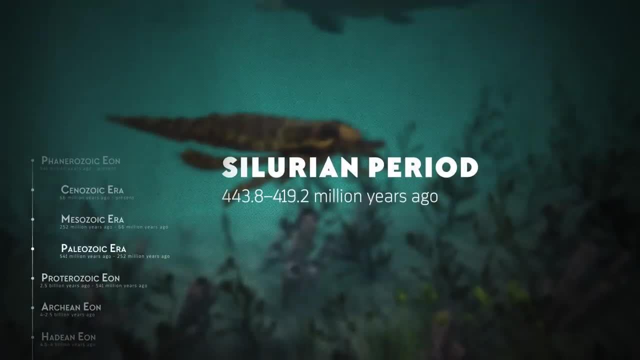 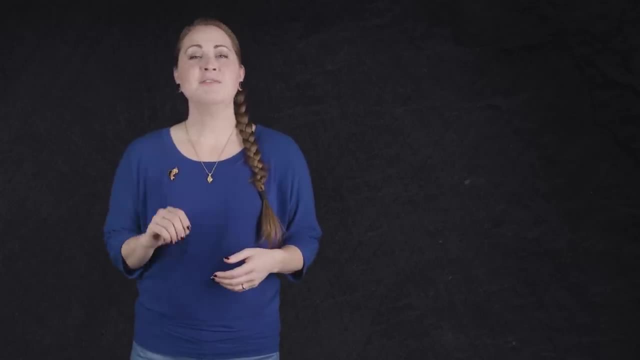 of the next period, the Solarian Life was able to recover once again in the Solarian. this time, as the climate gradually warmed, Plants, for example, started to spread over the land. Fossils of early vascular plants like Cucsonia first appear in rocks from this period as 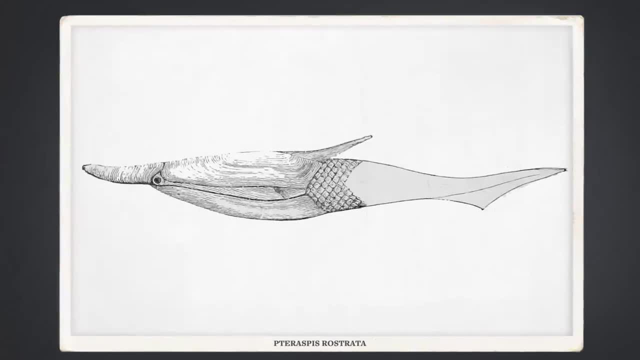 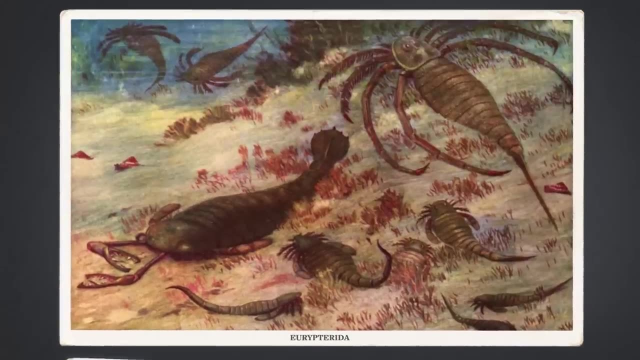 do the first fossils of terrestrial fungi. The Jollis ostracoderms were still the most common swimmers in the sea, and they developed spines and horns likely to protect themselves from carnivorous sea scorpions, the Eurypterids. 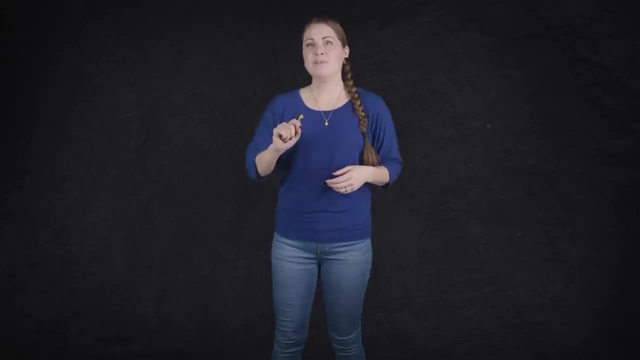 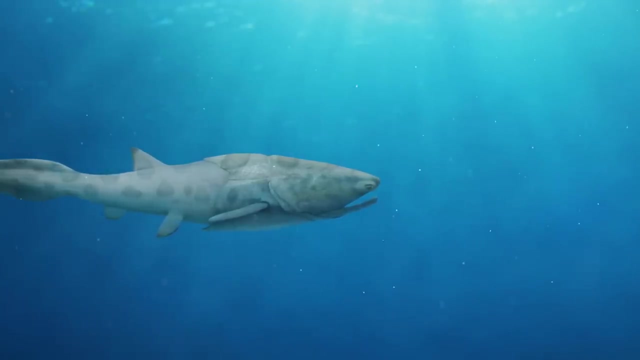 But by the end of the Solarian, 419 million years ago, a new type of fish learned to bite back. Jawed fish like Entelodnathus appeared in the seas, equipped with biting power that allowed them to tackle prey that the Jollis fish couldn't handle. 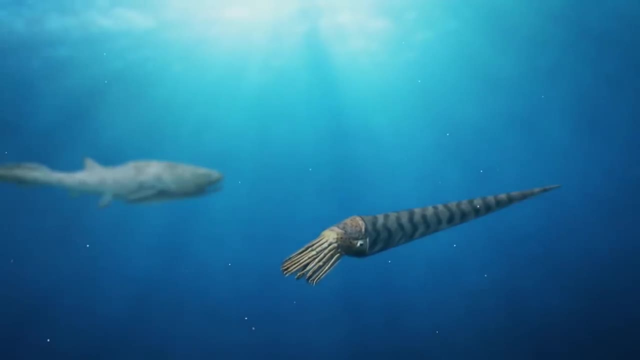 And the Solarian drew to a close with its own relatively minor series of extinction events, likely brought about by the drops in sea level that caused many bottom-dwelling species, particularly seabirds, to die, But the Solarian continued to survive. It was only a matter of time before the Eurypterids and cephalopods died out. The period that followed the Devonian was when fish began their takeover of the seas. During this time, the earliest sharks make their appearance. 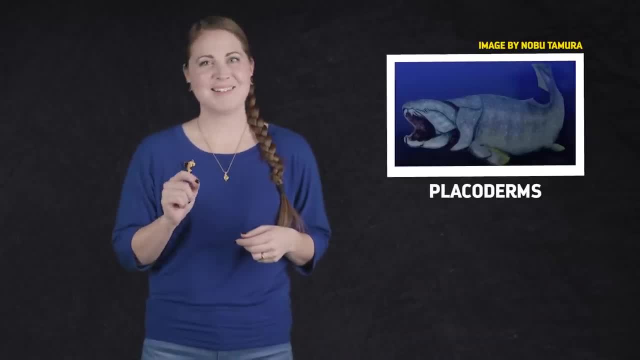 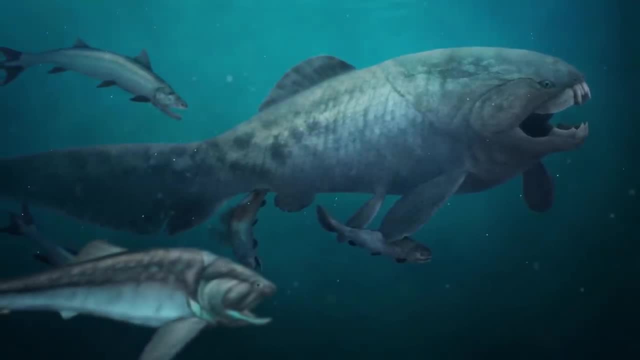 But the true kings of the Devonian were another kind of fish, the Placoderms. The largest of these jawed armored fish filled the niches we associate with whales and sharks today, including filter feeders like Titanichthys and apex predators like Dunkleosteus. While the Placoderms were conquering the seas, things were getting even more crowded on land. Arthropods really started to diversify with the first insects and terrestrial arachnids. emerging Trees also arose at this time, forming a canopy above the arthropods and these Devonian forests. 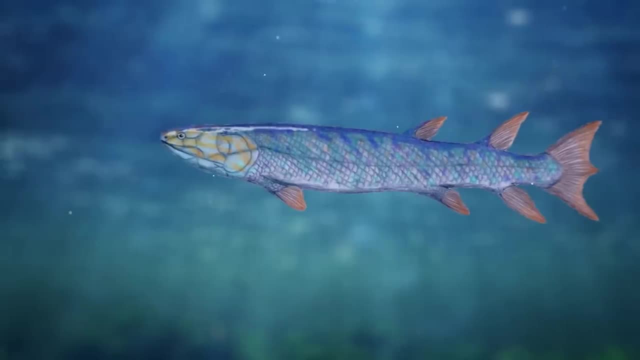 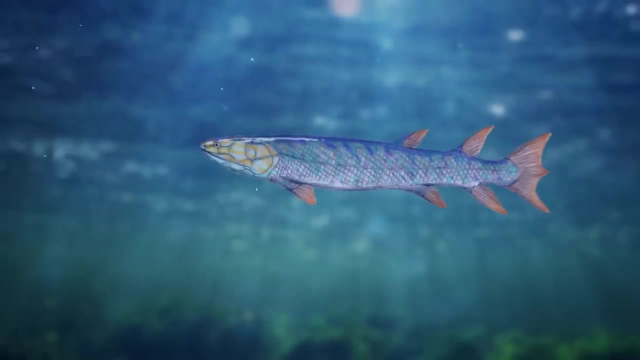 became the first major terrestrial ecosystems on Earth. Meanwhile, back at the water's edge, relatives of lobe-finned fish had adapted to spend more time in the shallows, pulling themselves along muddy shorelines. Then, 397 million years ago, descendants of these critters finally hauled themselves on. 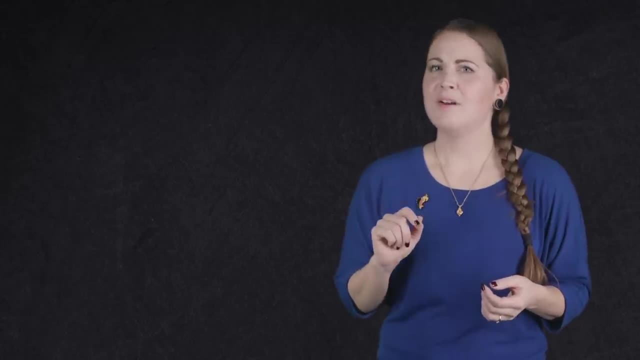 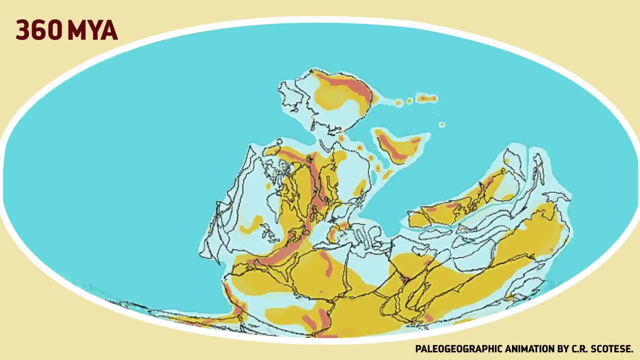 land for the first time. No skeletons of these ancient pioneers are known, but footprints in Poland show evidence of these very first tetrapods, animals with forelimbs. By the late Devonian 365 million years ago, tetrapods had made their way across the entire. 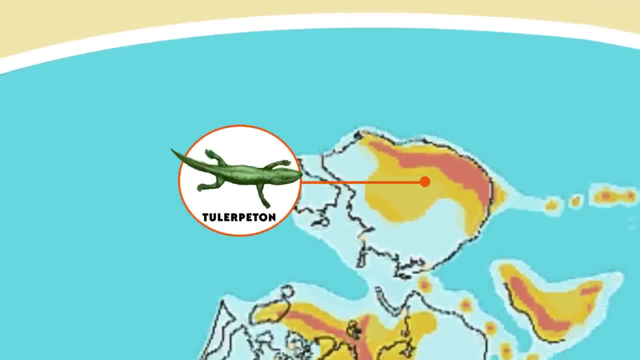 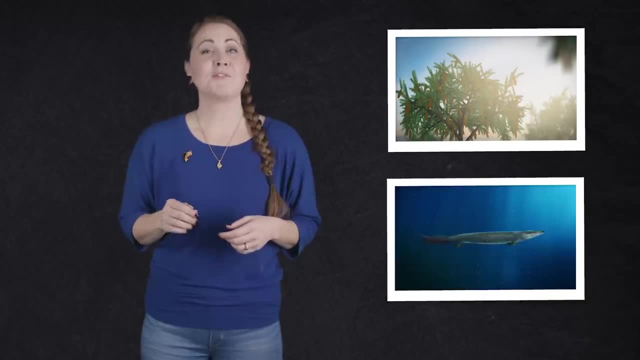 globe, from Acanthostega in Greenland to this dude in Russia. So the Devonian produced the first complex land ecosystems, while also seeing vertebrates take center stage in the oceans for the first time. But the period ended in, you guessed it, another mass extinction. This one took place from 378 million years ago. This one took place from 378 million years ago. This one took place from 355 to 358 million years ago and came in at least two phases Together. these events are known as the Late Devonian Extinctions, and they seem to have 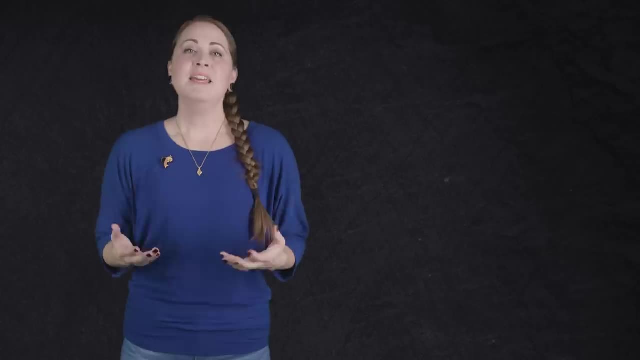 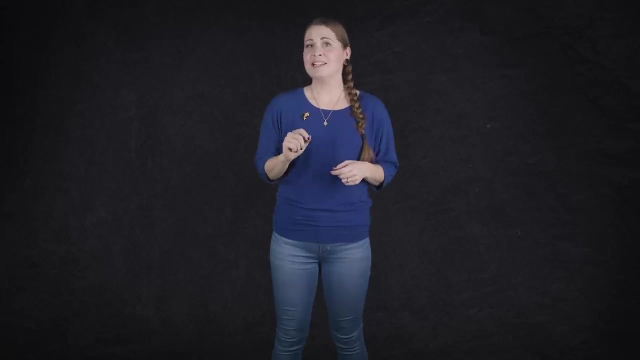 been caused by a series of drops in oxygen levels in the seas. By the end of the Devonian, many trilobites and all of the armored placoderms had vanished from the world's oceans. Luckily for us and other land animals, at least some early tetrapods survived into the 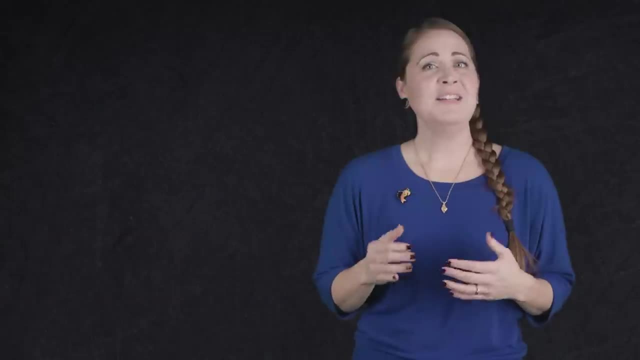 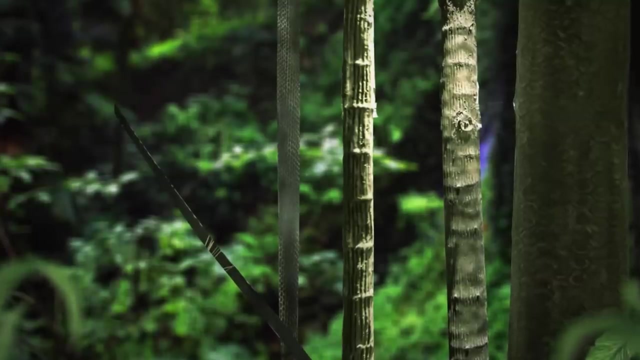 next period, the Carboniferous. But these creatures lived in a very different world from the Devonian. This time, oxygen in the atmosphere ramped up, The atmosphere ramped up and this, along with a humid, warm climate, allowed dense. 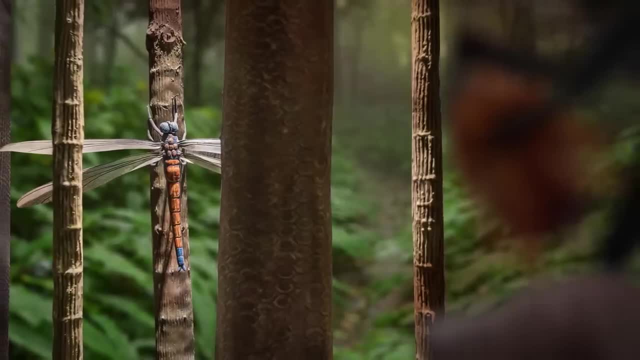 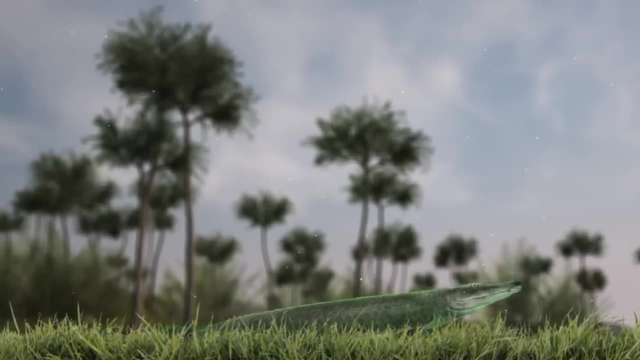 forests and swamps to spread across the continents. All that oxygen was also a plus for the arthropods, which got huge in the Carboniferous. But the bigger news was a major change among the tetrapods. Previously, all tetrapods laid their eggs in water. 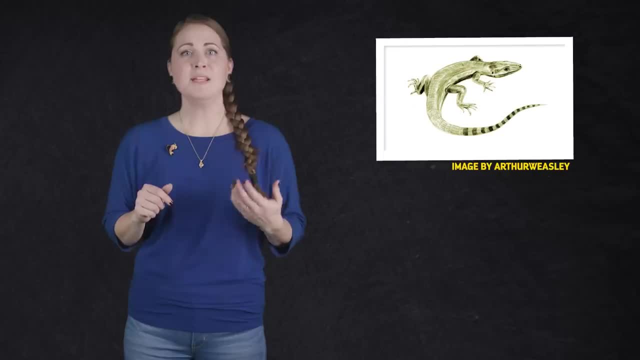 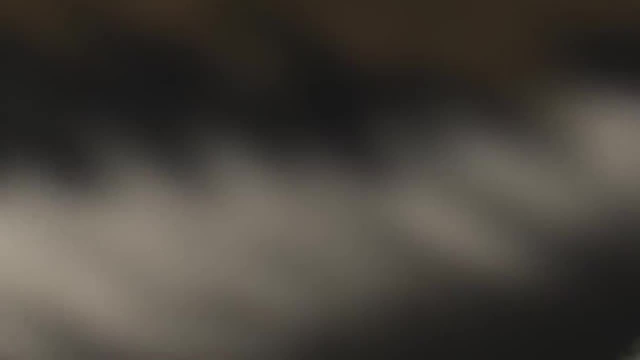 But around 340 million years ago, a group of tetrapods called amniotes began laying their eggs with shells that protected them from drying out, And this turned out to be a crucial adaptation, because it was around this time that the continents began to merge into a single supercontinent. Eventually, over millions of years, it would become Pangea. This landmass was so big that it was impossible for moisture from the ocean to reach inland. The result: A severe drop in humidity and temperature that wiped out much of the Carboniferous forest. 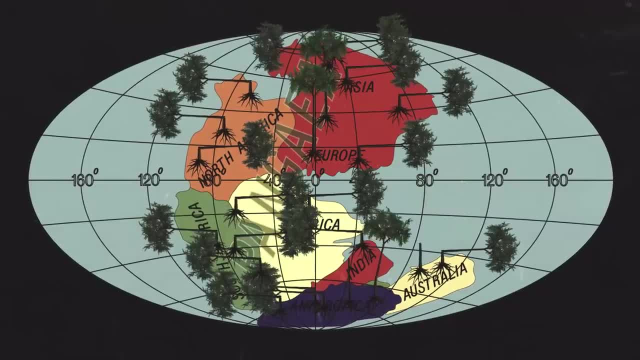 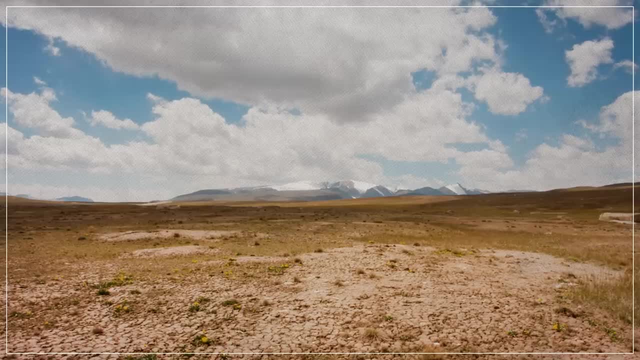 about 305 million years ago. It's known today as the Carboniferous Rainforest Collapse. By the end of this period, about 290 million years ago, much of the forest was covered by a giant desert at the heart of the continent, with extensive glaciers in the southern hemisphere. 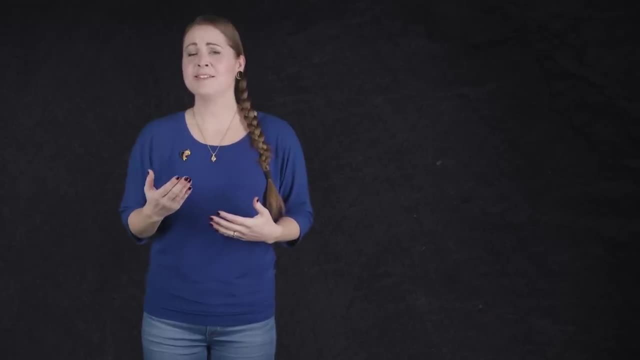 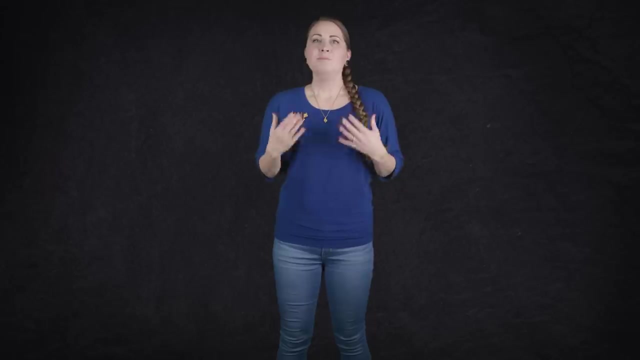 These arid wastelands would have been uninhabitable for early tetrapods, but not for the amniotes, And they rapidly split into two major groups, the reptiles and the synapsids, And both groups spent the last period of the Paleozoic the Permian, spreading across Pangea. 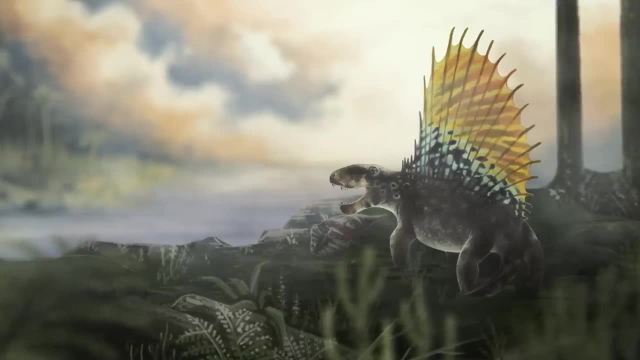 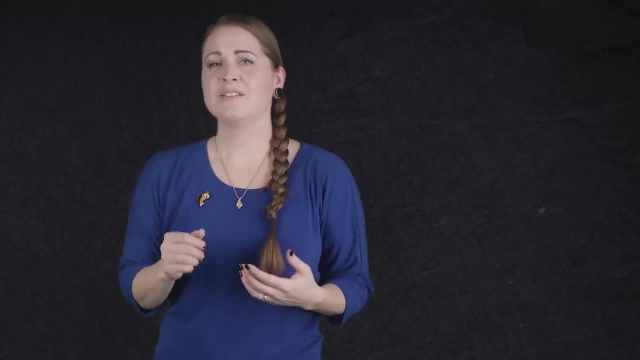 The synapsids were actually stem mammals and they were survivors, producing the first large terrestrial herbivores like Dimetrodon, But as time went on they became extinct. As the Permian went on, the climate got hotter and drier. Stem mammals and reptiles alike were forced to adapt to even harsher conditions. On the reptile side, there were cattle-sized herbivores like Pariasaurs. Meanwhile, stem mammals grew even stranger with the saber-toothed Gorgonopsids hunting. 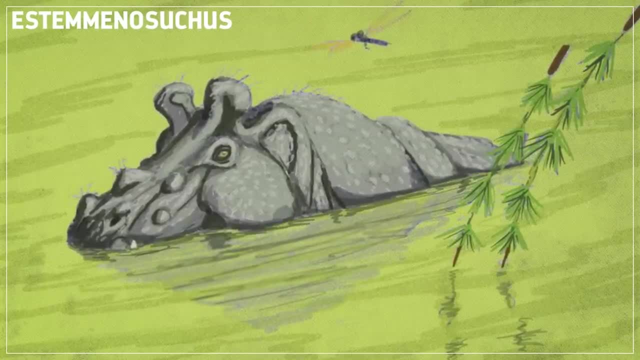 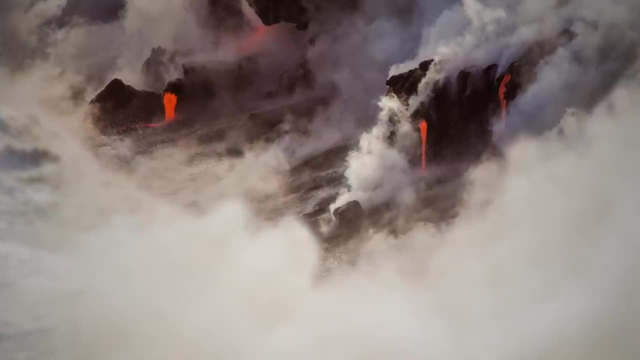 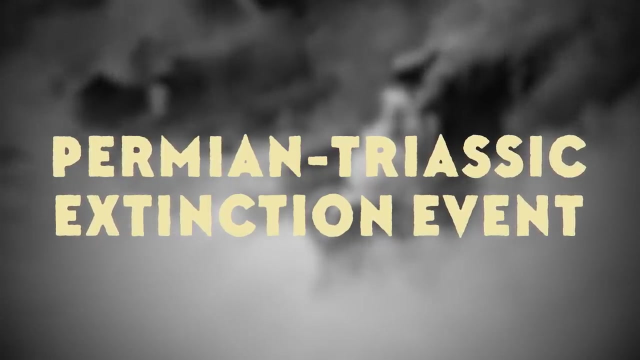 hippo-like omnivores with weird head ornaments, like Asteminosuchus. But this Permian safari park came to a terrifying end 252 million years ago. It was probably caused by a combination of volcanic activity and climate change, but the result- the Permian-Triassic extinction event- nearly spelled doom for life on Earth. 96% of marine species, including many sharks, fish and all the trilobites, were wiped out On land, the stem mammals and reptiles suffered as well, with a 70% loss of terrestrial species. So it began with an explosion of life, but the Paleozoic ended in near-apocalypse. 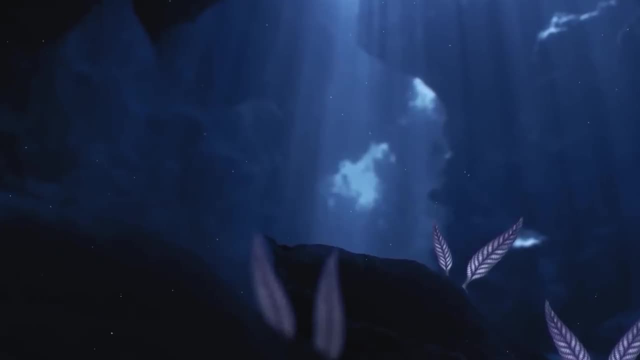 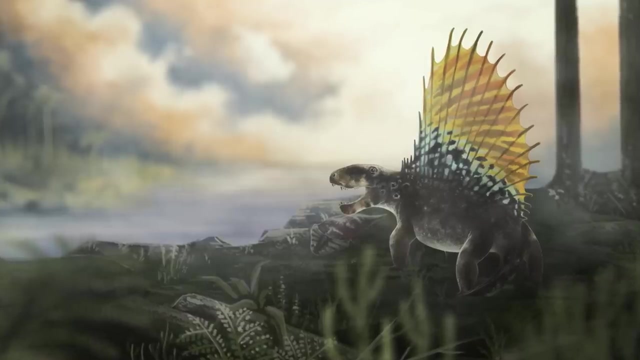 And while life started out in this era as simple small marine organisms, by its end life had conquered the oceans, taken the very first steps on land and spread to the most inhospitable corners of our planet. So, yes, it was not exactly a heyday of charismatic megafauna, but it's no overstatement to say 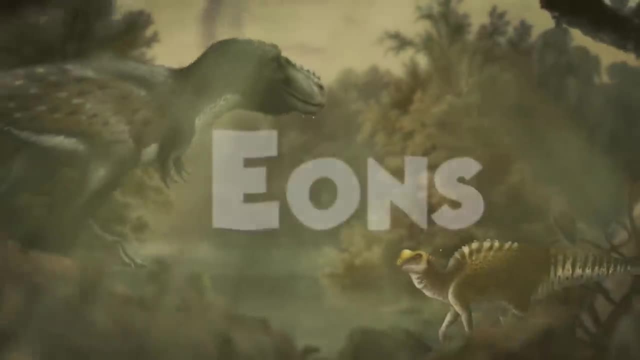 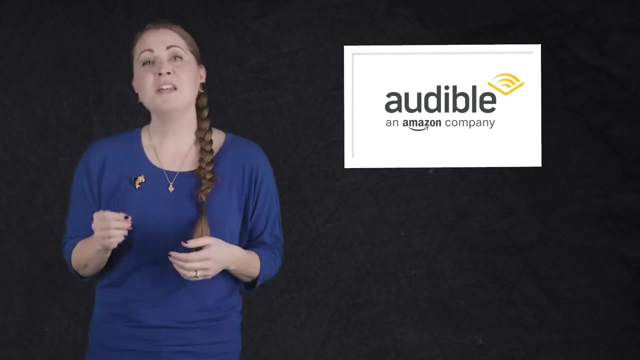 that the Paleozoic era made life what it is today. Thank you to Audible for supporting PBS Digital Studios, And right now Audible is offering Eons viewers a free 30-day trial. Just go to audiblecom slash eons to access all of their audio titles and programs. 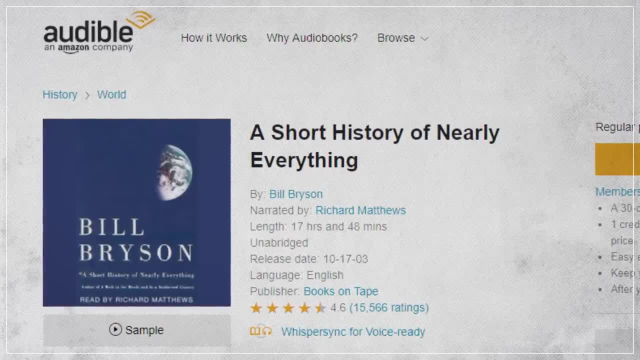 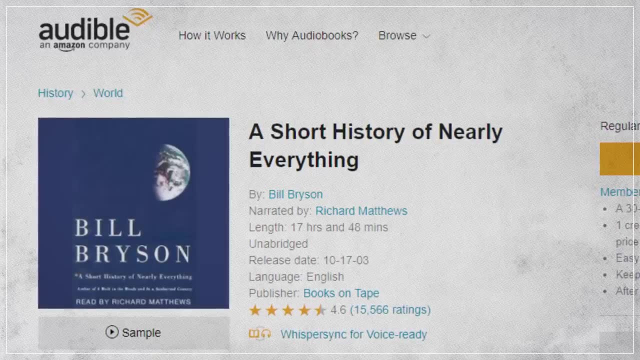 This week. I wanted to tell you about a short history of nearly everything which is Bill Bryson's wry. take on well, a lot From the Big Bang to civilization. Bryson is funny, informative and insightful. Sometimes science writing can get a little heady and Bryson does a wonderful job at 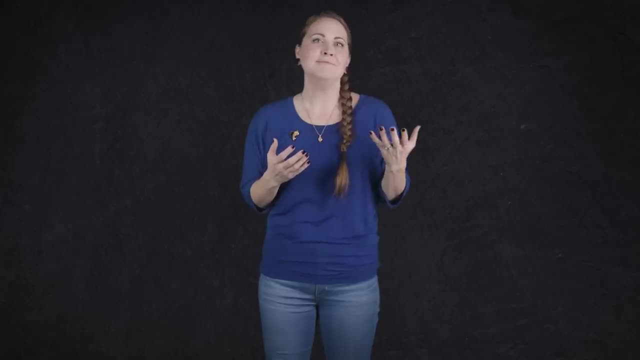 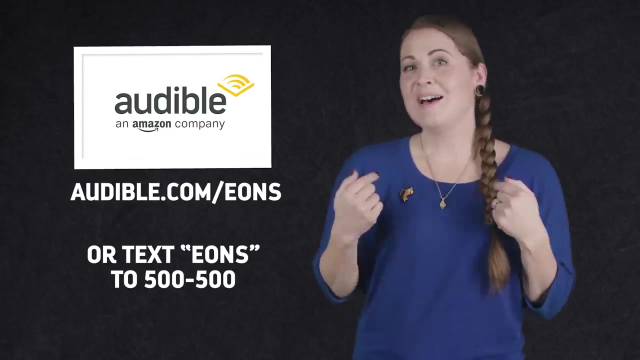 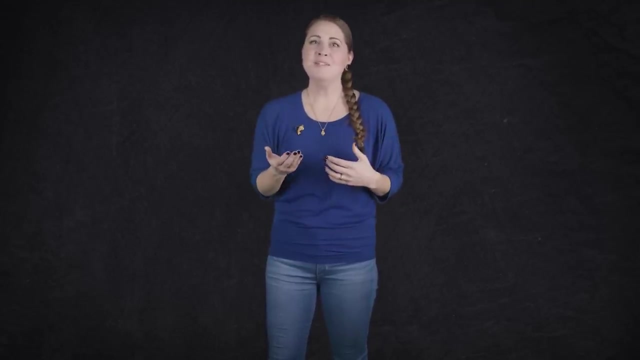 both making it all much more clear and making it fun and funny. You can check out this title and many others by going to audiblecom: slash eons. Make sure you use this link to help us out and to get your membership trial. And if you are really into dinosaurs and other big, scary creatures, then by all means watch. 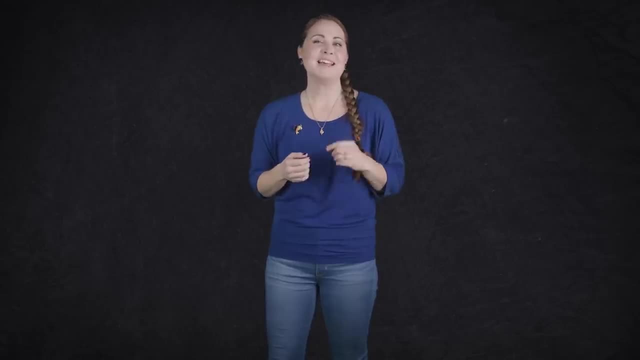 out for an episode coming soon about the next chapter in life's history, the Mesozoic era. But for now, thanks for joining me And, as always, I want to know what you want to learn about, so leave me a note in the. 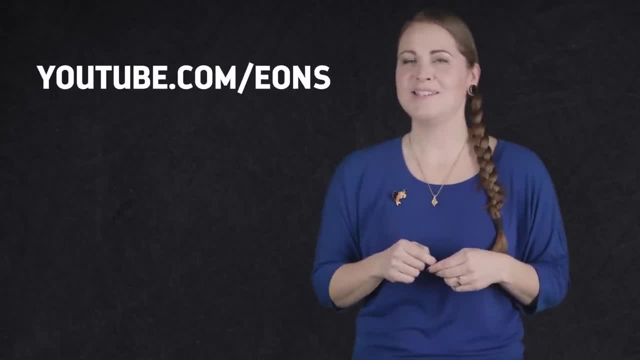 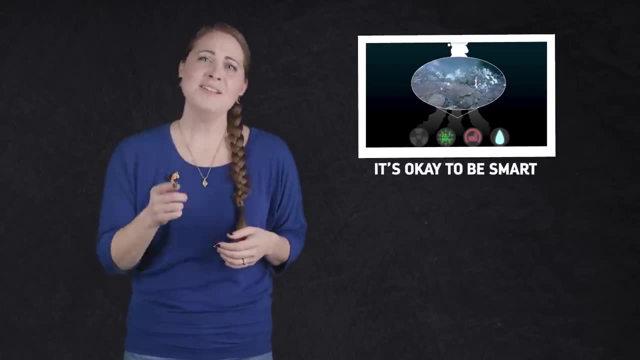 comments below And be sure to go to youtubecom. slash eons and subscribe. Now are you feeling smarter already? Well, continue to flex that brain muscle and check out. It's OK To Be Smart. They have an awesome episode that explores the most extreme life on Earth, like my favorite. 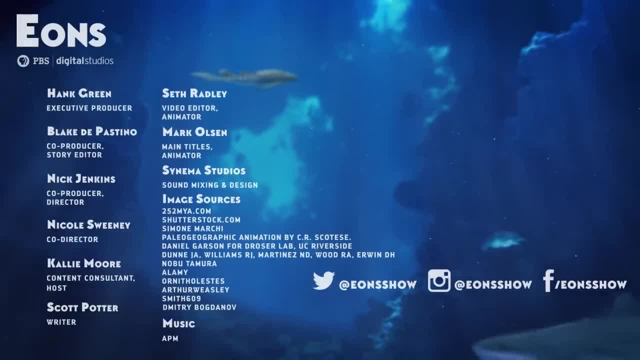 microfauna, the tardigrades, And I'll see you in the next one.